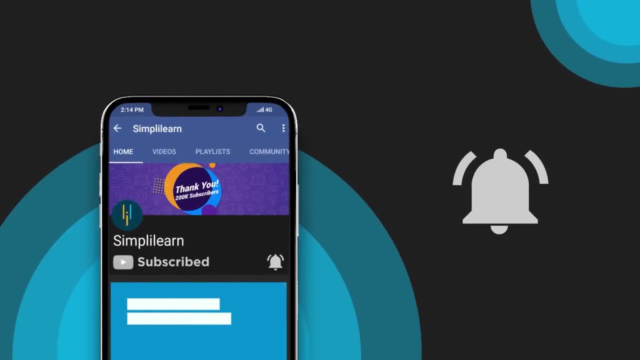 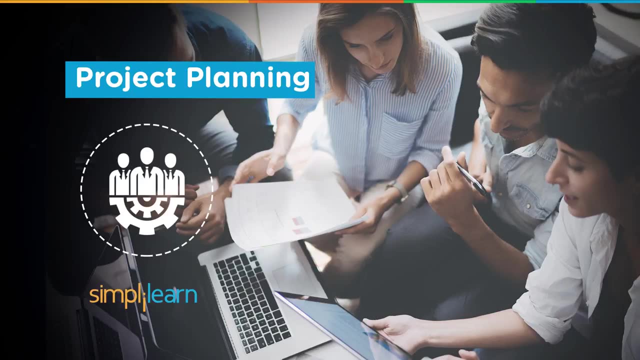 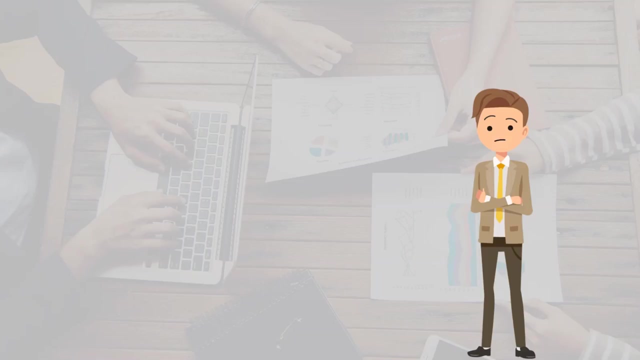 Hi guys, my name is Ishan and I welcome you all to this session of project planning. Today we will be learning about different aspects of project planning, But before we begin, let's have a look at an incident. Here's Max, an assistant project manager, who looks tensed. 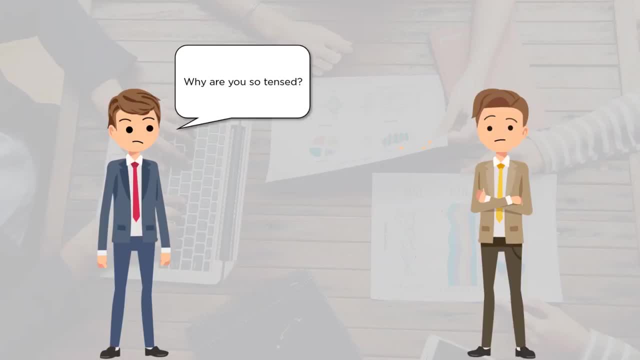 and is pacing around the room. Then Jack, a project manager who works with him, walks into the room and asks him why does he seem so tensed? To which Max replies he is facing difficulty in estimating the budget. Jack responds it might be because he is not planning the project properly. 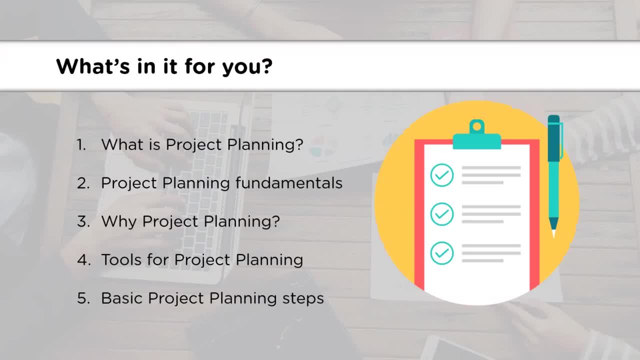 Jack reassures Max and begins to tell him about project planning. So today we will be learning about what is project planning and check out the fundamentals of project planning. Then we will see why project planning is so essential for a project to be successful. After that we will check the. 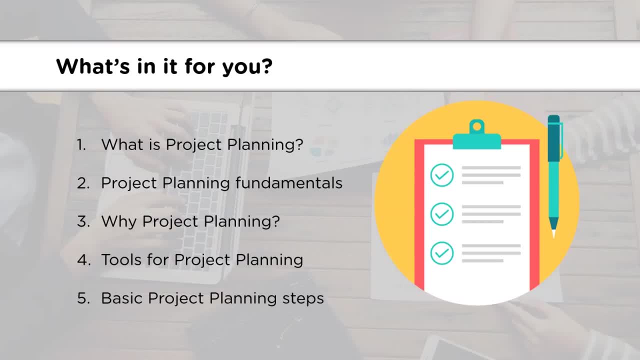 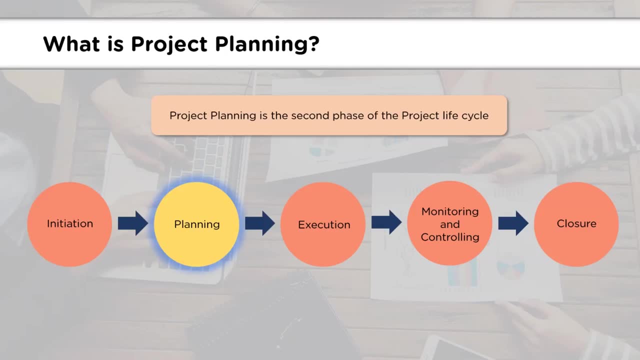 tools for project planning and, finally, we will have a look at the steps for project planning. So, without any further ado, let's begin with. what is project planning? Project planning is the second step or phase of the project life cycle. Project life cycle has five different phases, from initiation to closure. 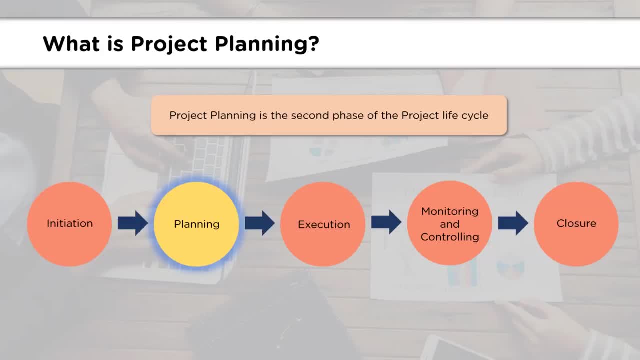 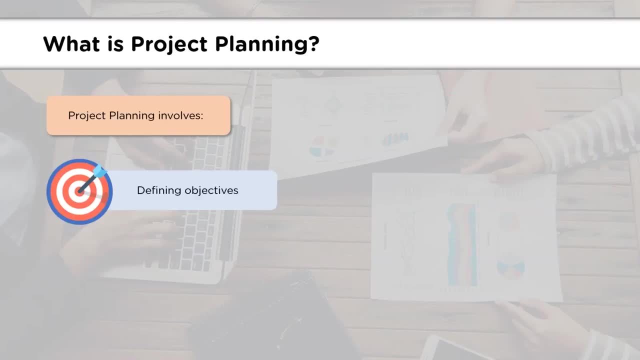 Today we will be learning about this phase that comes immediately after initiation, in which the project plan is documented and further requirements are defined. Project planning includes the following things. The first and foremost thing is describing the objectives or outputs we are expecting the project to yield. Second we have is the elaboration of the scope to make sure. 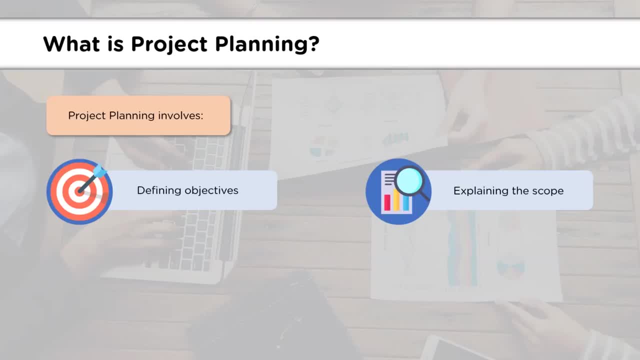 that the project is going to be successful. So let's get started. First, we have to understand what the project is all about and what all can be expected from the project. The third step we have is forming a schedule. This schedule is important to run or perform different. 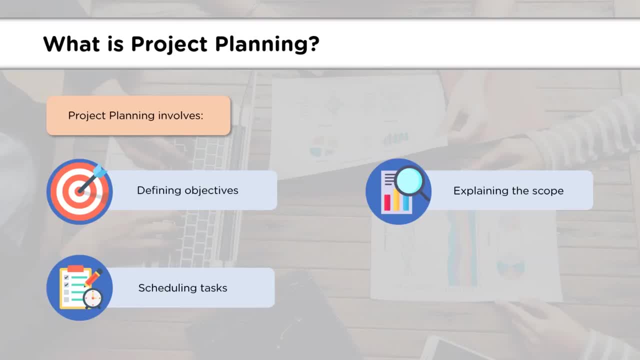 tasks of a project, each task having its own start date and end date. This helps the project to finish in the scheduled time and limit. Lastly, we have making and generating progress reports in which all that went during the tenure of the project is documented. This helps in evaluating the project. 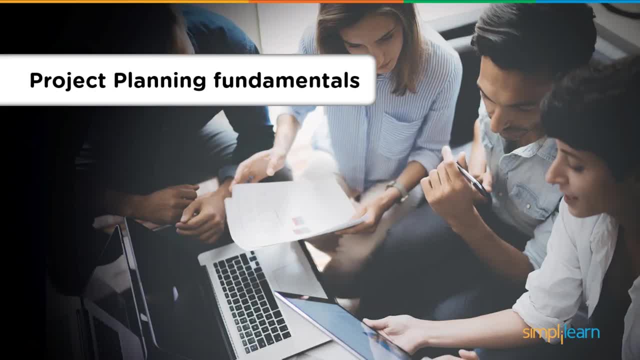 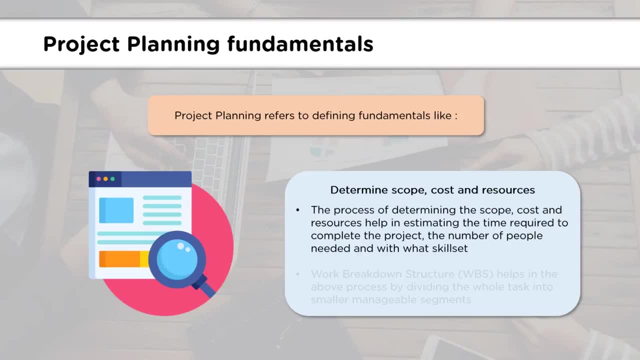 and helps in the forthcoming projects. Now let's have a look at the project planning fundamentals. The first fundamental that we have is the determination of scope, cost and resources. The determination helps us in having a rough estimate about the time that is required to. 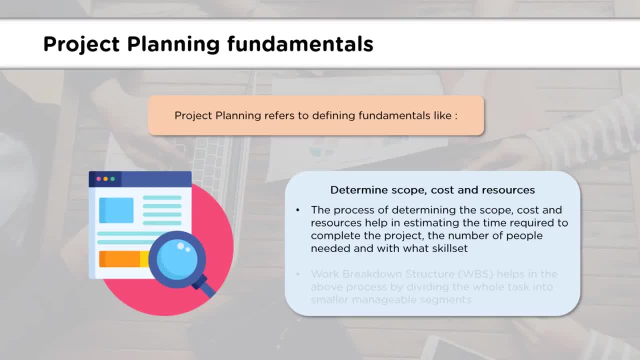 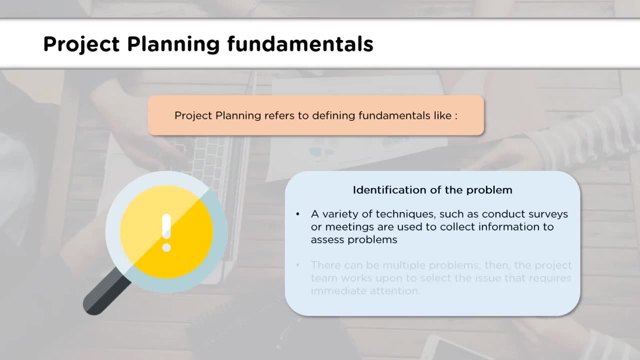 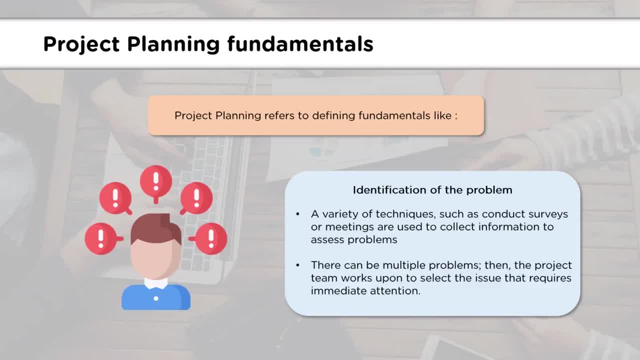 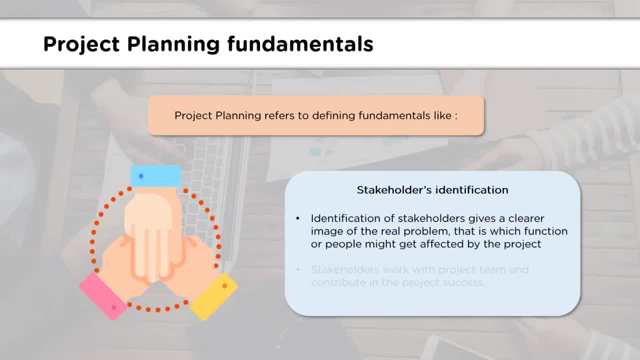 Then comes Identification of Stakeholders. When we can identify the stakeholders, we can know who all will be affected and in what way, which helps us having a better understanding of the project. Stakeholders may be anybody. They may be the part of the project team, or project managers or customers. 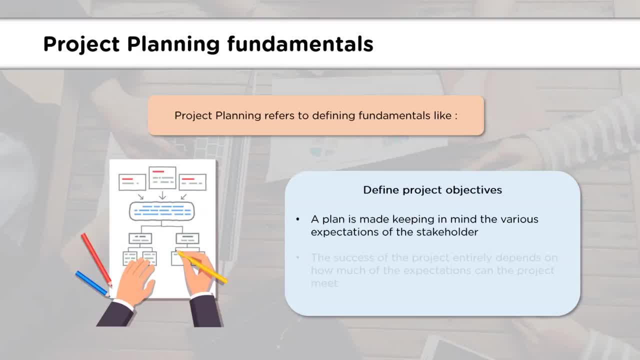 They help during the project and contribute to its success. Then the last fundamental we will discuss is Defining Project Objectives. A project plan is made keeping in mind the requirements of the project team and expectations of the stakeholders. If the project team can meet the expectations of the stakeholders, then only we can say: 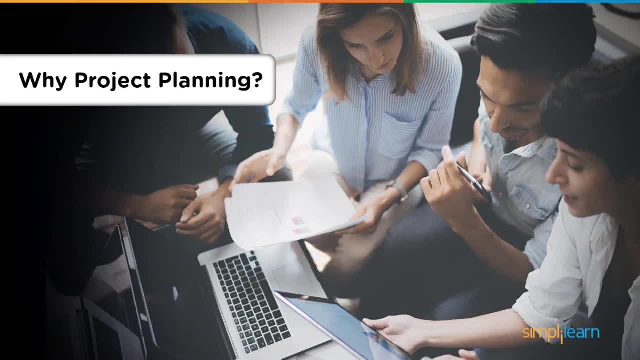 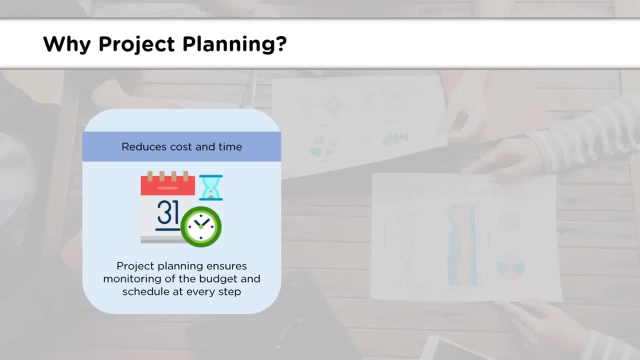 that the project is successful. Now, when we know about project planning and its fundamentals, it's time to see why project planning is so important. Project planning reduces the cost and time of the project, as every step is monitored and optimized in the best possible manner. 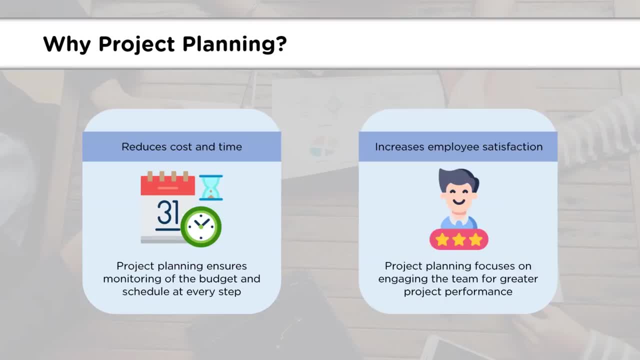 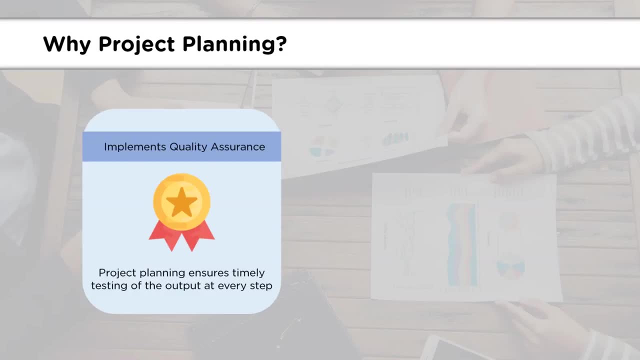 Project planning increases the cost and time of the project, as every step is monitored and optimized in the best possible manner. Project planning reduces employee satisfaction, as every employee who is a part is engaged in the team for improved project performance. Project planning helps in the implementation of quality assurance as the output of every 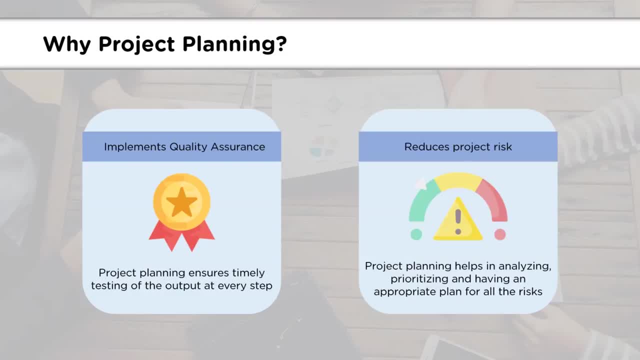 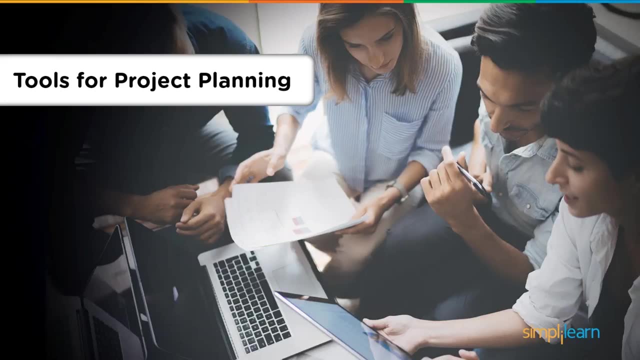 step is duly tested. Lastly, project planning helps in reducing project risk, as planning helps to analyze, prioritize and deal with that risk. Moving on, let's have a look at the tools for project planning. The first tool that we have is a Gantt chart. 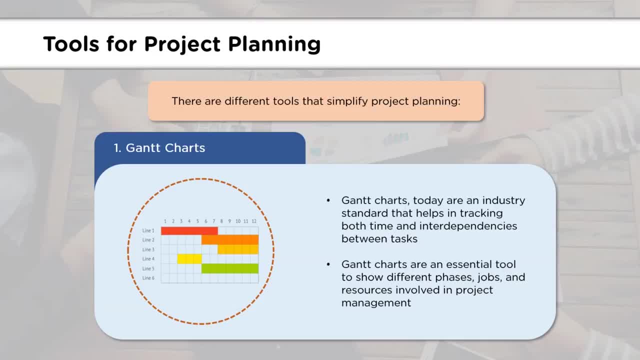 Today, Gantt charts are one of the most popular project management tools. They help in tracking the status of the work at a personal level. They help in tracking the status of the work at a personal level. They help in tracking the status of the work and their activities, in particular time and 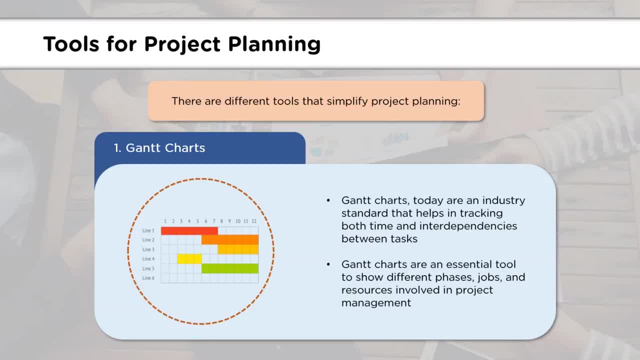 their independently on each other. Gantt charts help in showing different phases and steps involved in a project. The second tool that we will talk about is critical path method, or CPM. Critical path method helps in scheduling the project activities so that the project runs. 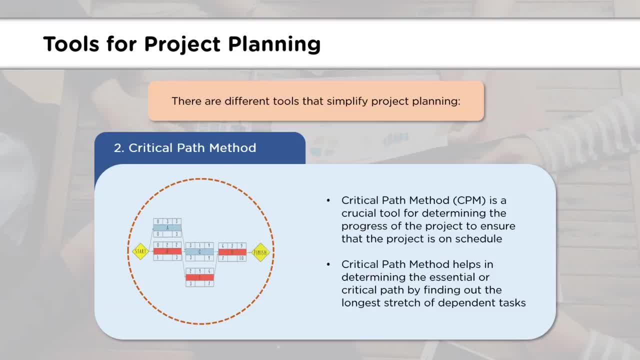 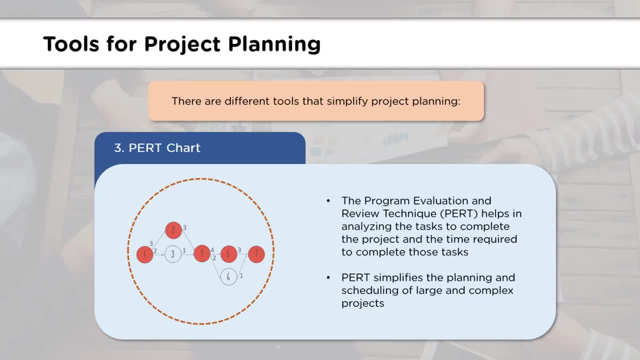 properly. The critical path method focuses on the longest stretch of dependent tasks and determines the time needed to complete them. The next tool is project evaluation and review technique, or PERT chart. PERT provides a graphical representation of the project's timeline. PERT provides a graphical representation of the project's timeline. 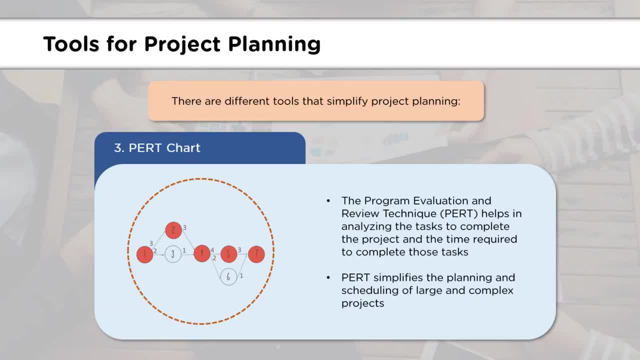 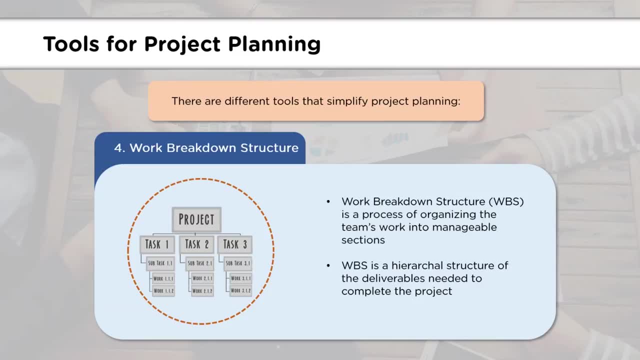 explaining the independencies of different tasks. This tool not only helps in making a schedule, but also helps in coordinating with all the team members. The fourth tool we will check is Work Breakdown Structure. Work Breakdown Structure is a very common tool that makes it possible for the team to break its work into manageable sections. 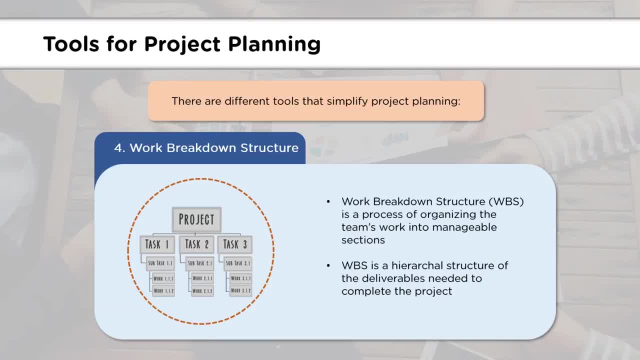 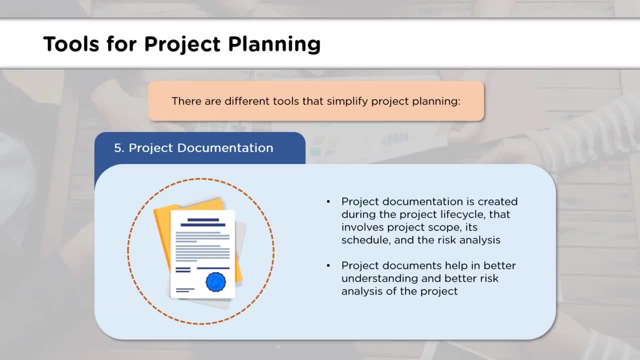 Work Breakdown Structure is a step-to-step process that helps in completing the project efficiently. The last tool we will see is Project Documentation. Project Documentation is an integral part of the project lifecycle. Project Documentation helps in understanding the mistakes done during the project and, more importantly, provides guidelines for the upcoming project. 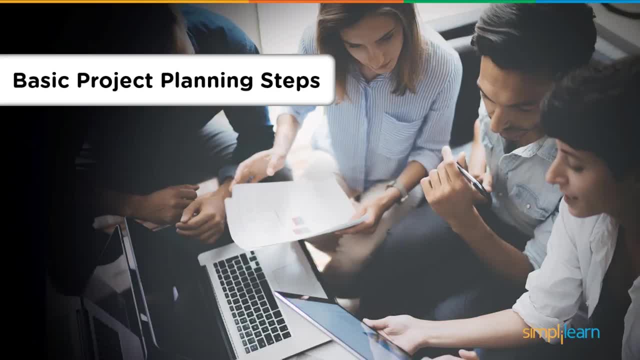 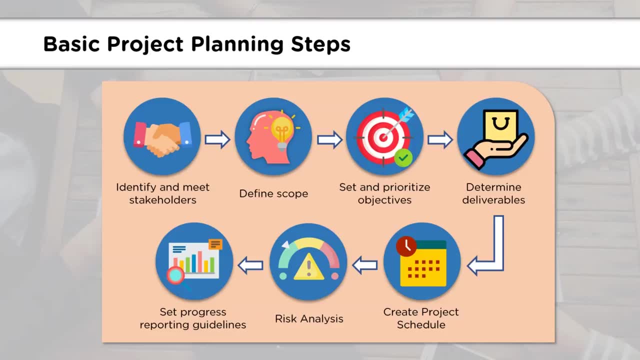 Now, when we know about different tools for project planning, it becomes essential that we know the necessary steps of project planning. There are seven steps in project planning. Let's have a look at each of them in detail. The first step is identification of stakeholders. 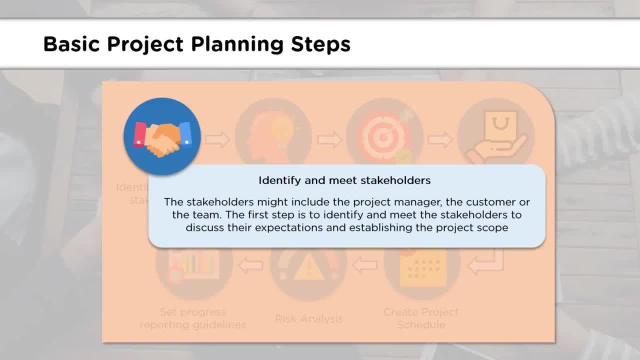 As we have discussed, stakeholders could be anybody. They could be a part of the team or a project manager or a customer. When we identify stakeholders, we can find out the expectations and requirements that are to be looked upon in this project. This gives us a clearer picture of the project. 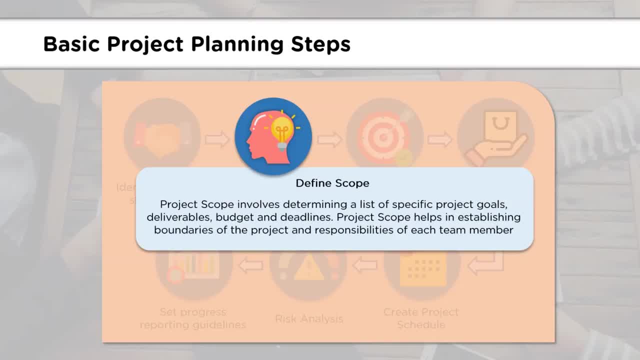 and helps in establishing the project scope. So the next step we have is defining the project scope. This helps in determining a list of specific project goals and deliverables that are to be achieved during the course of the project. After we have defined the project scope. 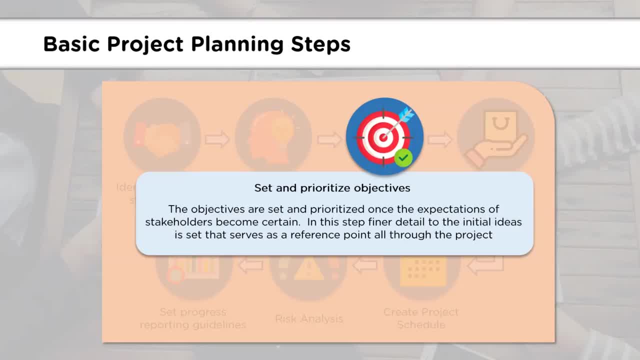 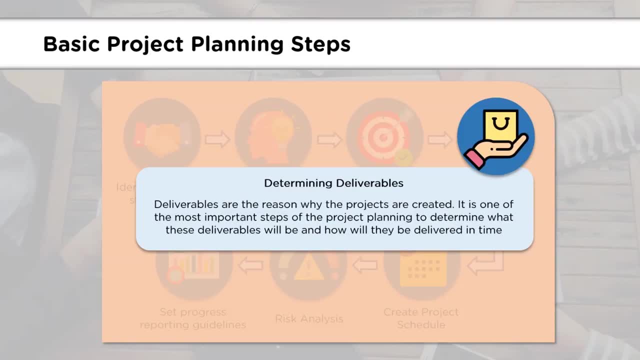 it is time to set project objectives and prioritize them. The initial ideas that were there before are now elaborated, and final steps to complete the project are defined. In the next step, the deliverables are determined. After all, project deliverables are the only reason.